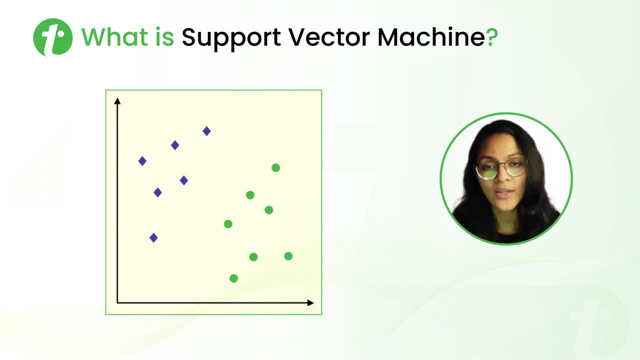 And we have plotted these data points on a graph. Now we have to separate them using a line. So how can we separate these two categories? We can separate these categories by drawing either of these two lines: red or green. Now the question arises: which line should we choose In this case? 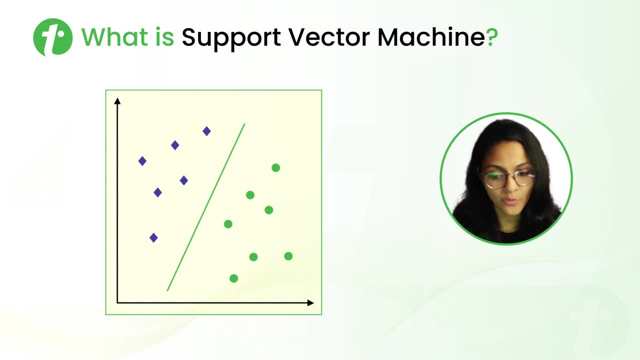 we choose the green line. Why is that? Before diving into that, let's understand some technical terms of the support vector machine. Let's understand some technical terms of the support vector machine. Let's understand some technical terms of the support vector machine. 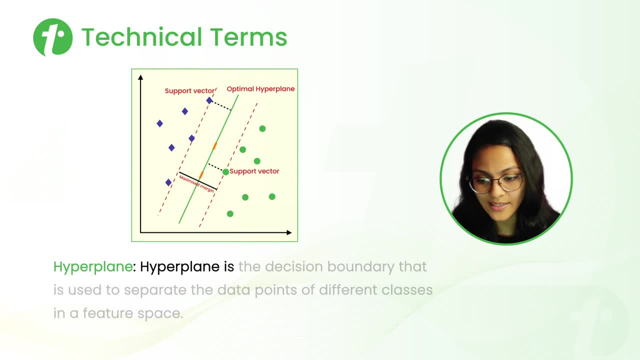 First is hyperplane. Hyperplane is the decision boundary that is used to separate the two categories. Next is support vectors. Support vectors are the closest data points to the hyperplane, which makes a critical role in deciding the hyperplane and the margin. 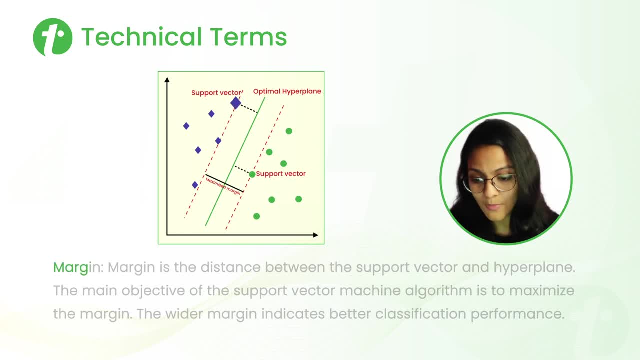 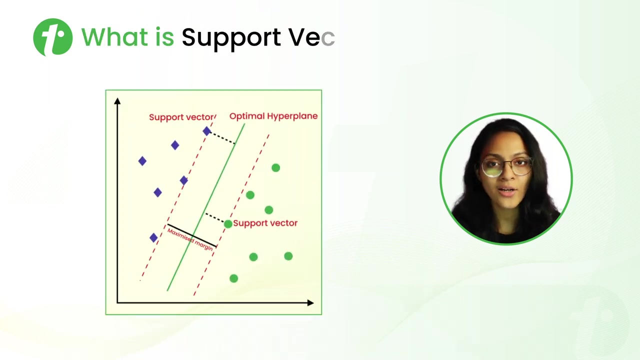 Next very important term is margin. So margin is the distance between the support vector and the hyperplane. The main objective of the support vector machine is to maximize the margin. The wider margin indicates the better classification performance. Now let's move to why we have chosen that green line as our hyperplane. We have hyperplane. 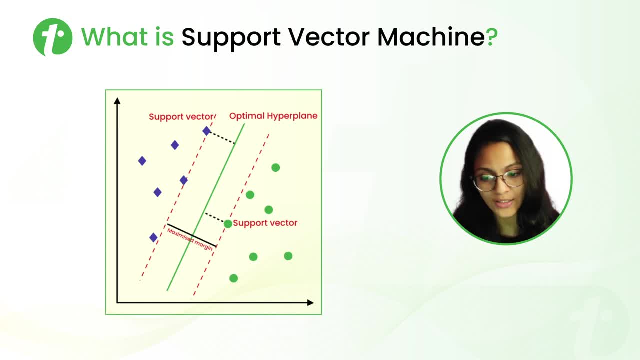 we have support vectors And the distance between the support vector and the hyperplane is called margin. For having the optimal hyperplane we need the maximum margin distance. So let's say this margin is our positive margin, D plus and this is our negative margin. 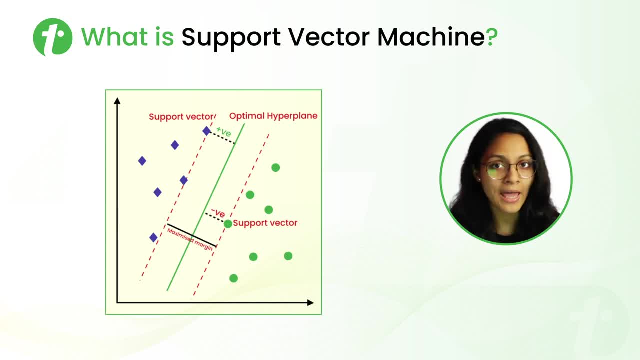 So we must have the maximum margin. that means the sum of D plus and D minus is maximum. So we can say that the hyperplane for which the margin is maximum is called the optimal hyperplane And that hyperplane gives us the best results. Now we had this kind of data set, So we use 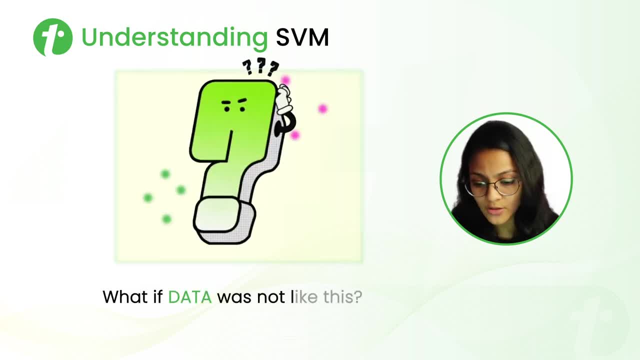 the hyperplane to segregate them. But what if the data was not like this? instead, it was like this: In this we have the data set of D plus and D minus. So we have the data set of D plus and D minus. 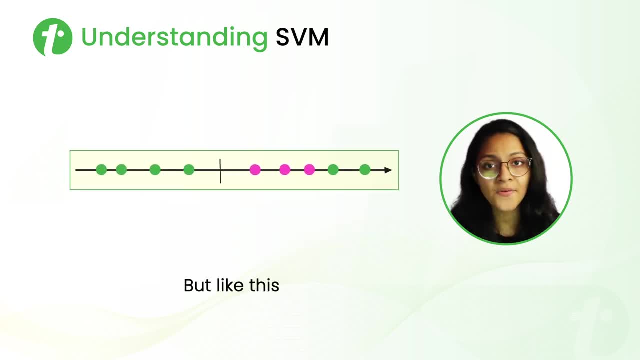 One kind of category falls under the another, And in this case we can't use the hyperplane to separate the two categories. So what we are going to do? So for this kind of data set, we transform our 1D plot to the 2D plot, And for the transformation, what we use is called